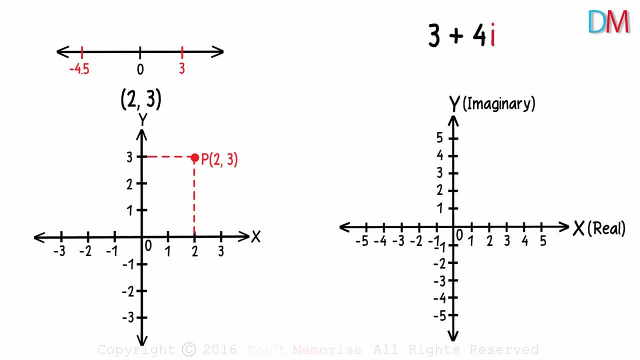 and the y-axis as the imaginary axis. So based on this, we can say that this complex number corresponds to the x-axis. So we plot the ordered pair 3 comma 4.. 3- the real part and 4 the imaginary part. 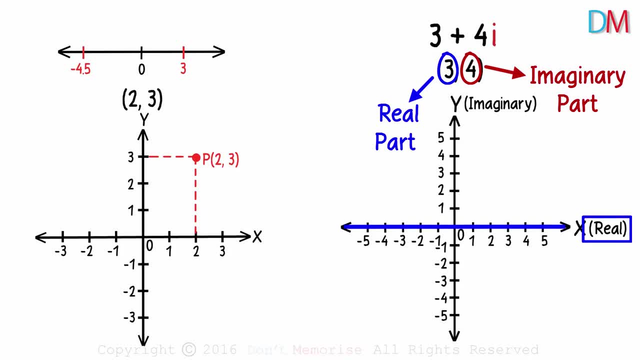 Remember the horizontal axis is the real axis and the vertical axis is called the imaginary axis. So 3 units right on the real axis and 4 units up on the imaginary axis will give us the position of the complex number on this plane. To plot the ordered pair of real numbers, 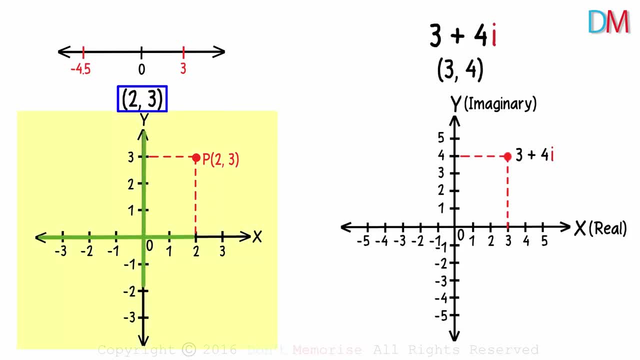 we use the xy plane, which had real numbers on both the axes. Do you remember what that plane was called? Yes, the Cartesian plane, And these coordinates were called the Cartesian coordinates. What is this plane called then? The plane in which the horizontal axis is the real axis. 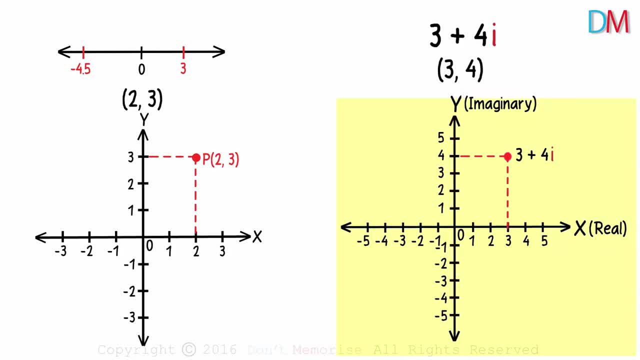 and the vertical one is the imaginary axis. It's called the Argand plane or the complex plane. It was Jean Robert Argand who is credited with development and elaboration on geometric representation of complex numbers and operations upon them. This assured him a place in history of mathematics. 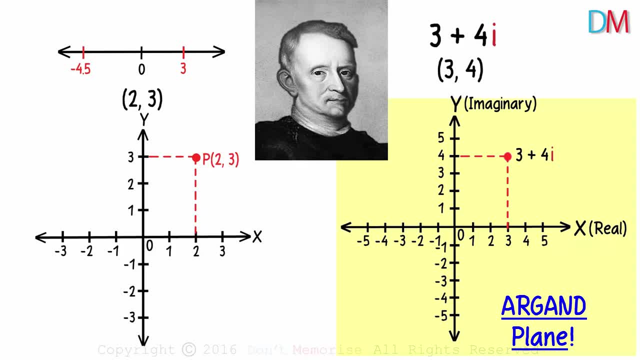 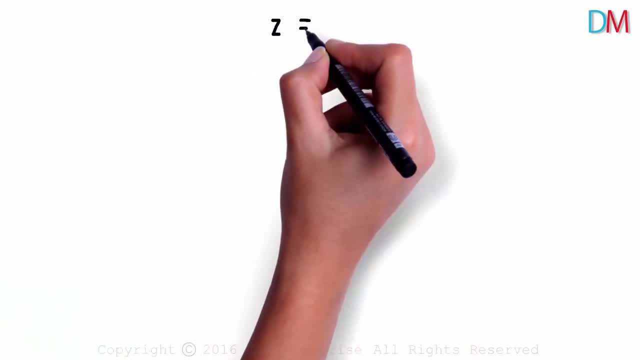 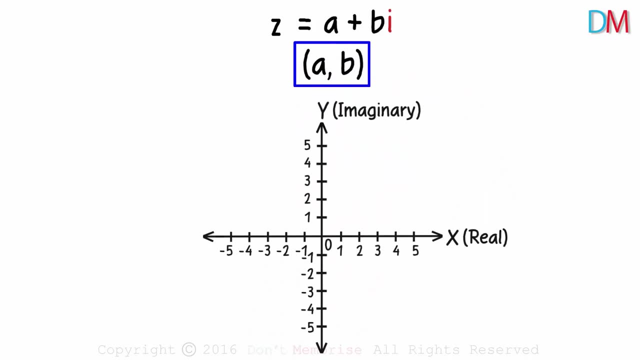 by calling his representation of complex numbers on a plane as Argand plane A. complex number z is equal to a plus ib is simply written as a comma b, And this can be represented on an Argand plane. Now what if the points lie on one of the axes of the Argand plane? 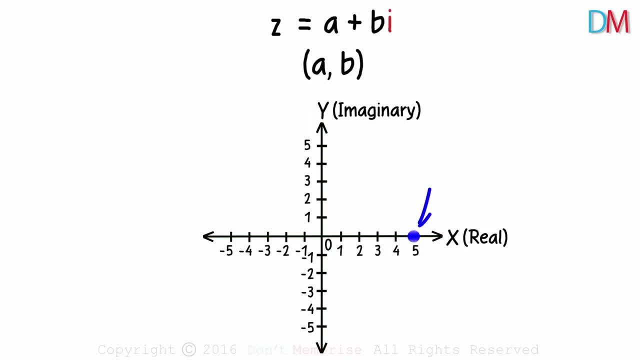 Say the point is here on the x-axis, This number will have only the real part. It can be written as five plus zero i. And if the point is here on the x-axis it will be negative: three plus zero i. And what if the point is here on the y-axis? 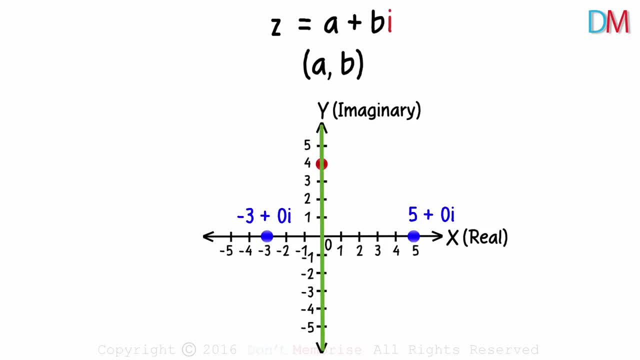 Every point on the y-axis will have only the imaginary part. So this point will be zero plus four i. Every point on the x-axis will have only the imaginary part. Every point on the y-axis corresponds to a complex number of the form a plus i zero.